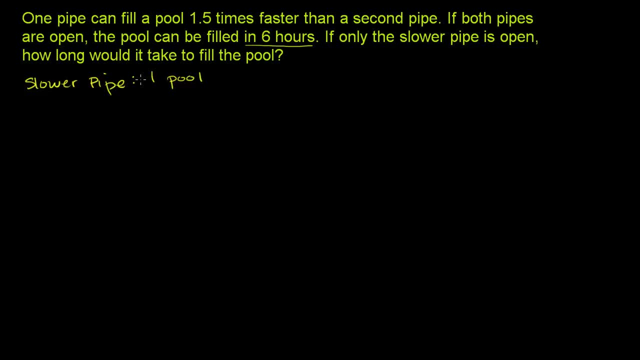 it can do one pool in T hours And I wanted to write its rate in terms of T, because that's what we're trying to solve for at the end. How long would it take to fill a pool? It takes T hours. It can do one pool in T hours. 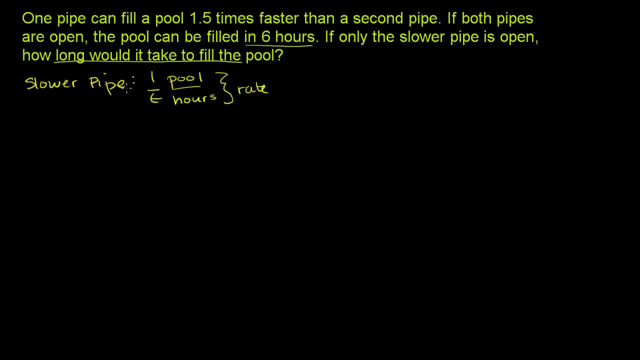 This is a rate over here. This is the rate at which the slower pipe can fill a pool. Now what about the faster pipe? Well, it tells us, one pipe can fill a pool one and a half times faster than a second pipe. 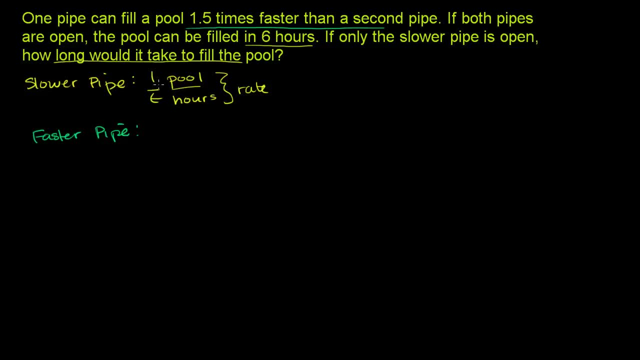 So the faster pipe can fill a pool one and a half times faster than a slower pipe. So if this can do one pool in T hours, the faster pipe can do 1.5 times that. It can do 1.5 pools. 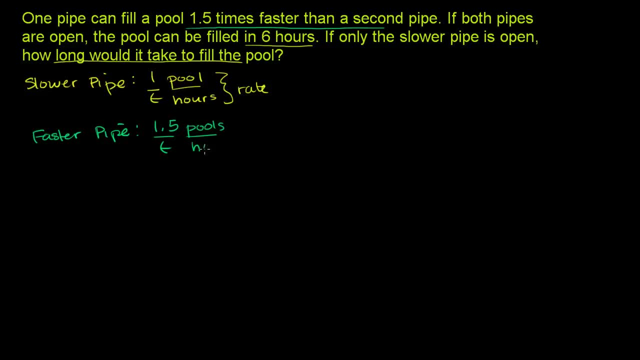 1.5 pools In T hours, Right In the same amount of hours, it can do one and a half times as much work, or one and a half times as much of a job. It can fill one and a half pools. 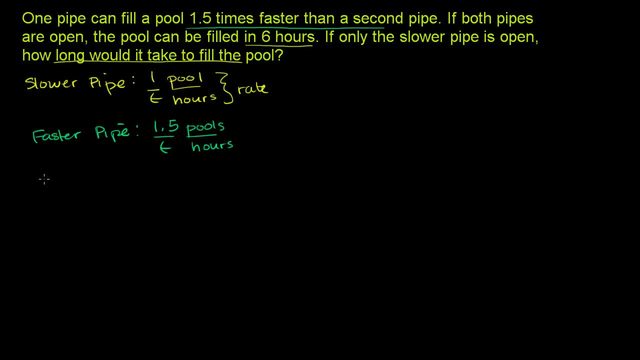 So how much can they do together? Well, together, Let me write this in orange, So let's think about it together. So together, what could they do? Well, let's just imagine that they're working together for T hours, So this can fill one pool in T hours. 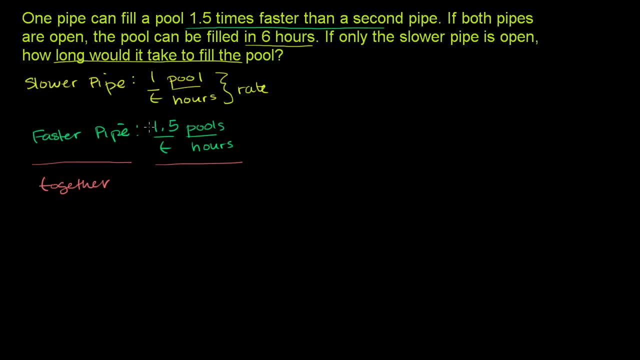 And this can fill one and a half pools in T hours. You can add these two things So you get so together. they can do one over T pools per hour, Pools per hour Or pool per hours. Sometimes the plural and singular gets a little bit messed up here. 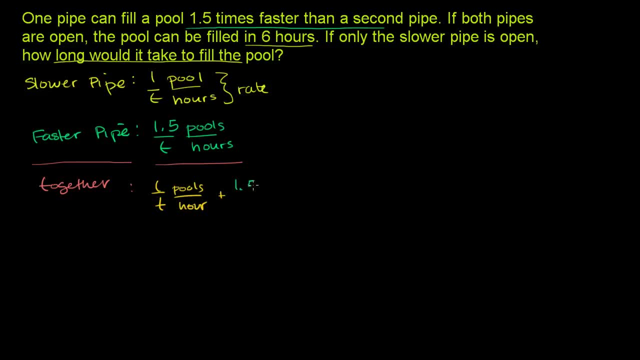 but hopefully you get the idea. Plus one and a half over T pools per hour, Plus one and a half over T pools per hour. So together, if you add these two things, they're going to be able to do, if you can imagine. 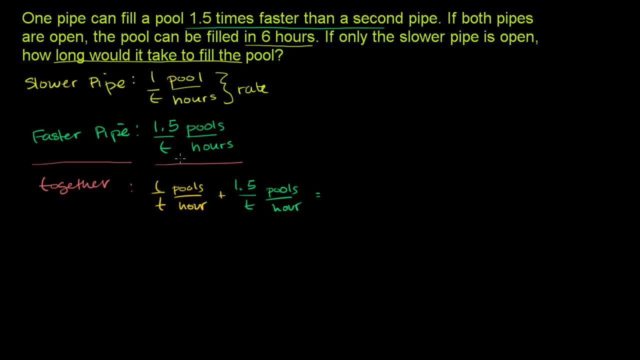 this guy can do one pool in T hours. this guy can do one and a half pools in T hours. Together they're going to be able. if you let T hours go by, together they're going to be able to do two and a half pools. 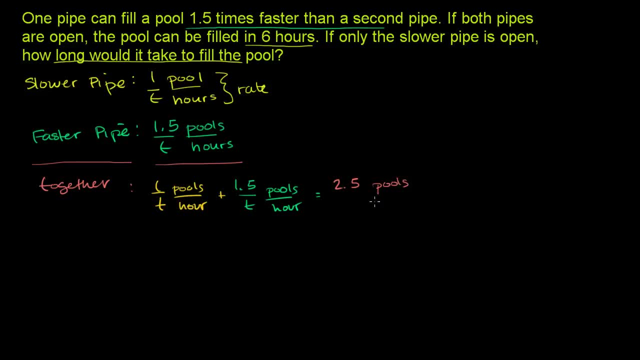 Two and a half pools Two and a half pools in T hours In T hours. And notice, the units are the same and you're really just adding one over T plus one and a half over T. You have the same denominator, so you can just add the numerators. 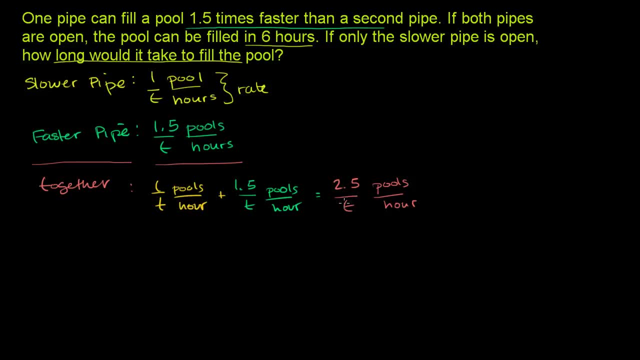 One plus one and a half gives two and a half, And it's very, very, very important whenever you're doing these rate problems is to always make sure that it's making sense. Okay, yeah, they can do more pools in the same amount of time. 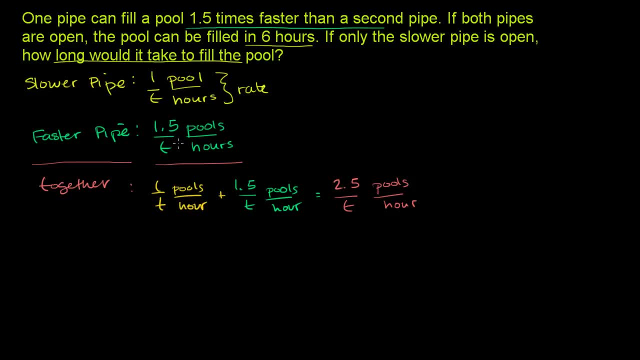 We've added the two, And I say that because sometimes, when you do this, you're tempted to do the inverse of these. You're tempted to say hours per pool, hours per pool, And then, when you add them, you will actually get more hours per pool. 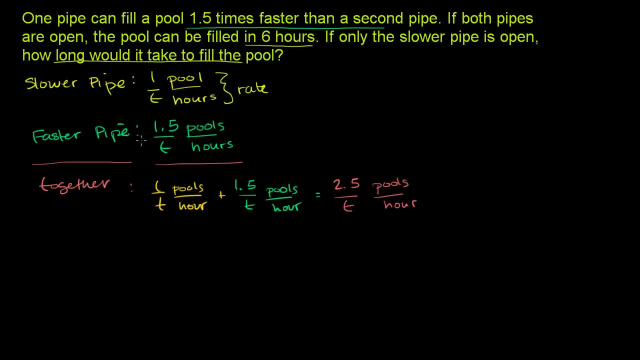 which is not intuitive even, Because if you have two things working together, it shouldn't take more hours per pool. You should get more pools per hour, And so that's a really important reality check whenever you're doing one of these rate problems. 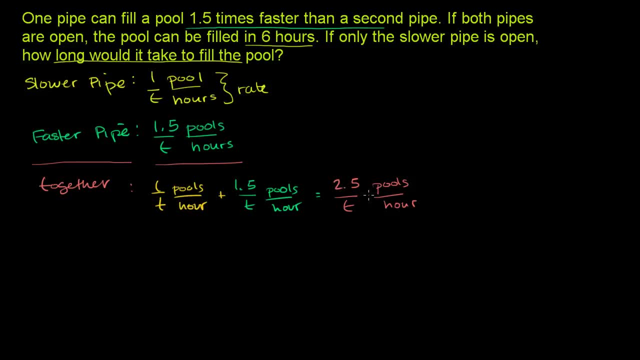 So anyway, if they're working together they can do 2.5 pools in T hours And remember the T was just how long the slower pipe takes to fill one pool. But they also tell us so this is their rate. 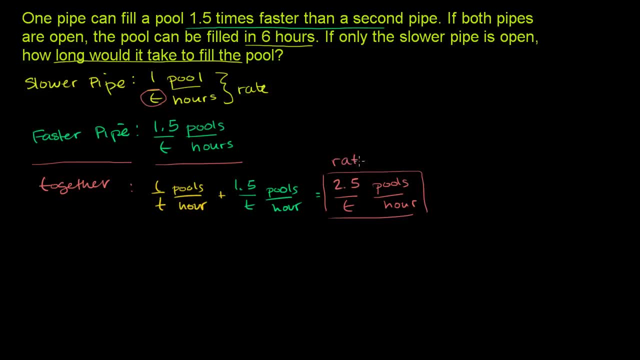 This is their rate. This is their rate at which they can fill pools, And then they tell us that at that rate, the combined rate together, if they work for 6 hours, then they can fill a pool. So you have the rate. 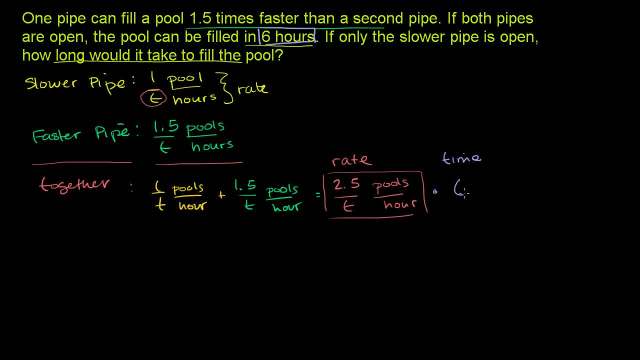 If you multiply it by the time, if you multiply it by 6 hours, you should get the amount of work they've done. And once again, this is not work in the physics sense, This is work in the everyday sense, the work of filling a pool. 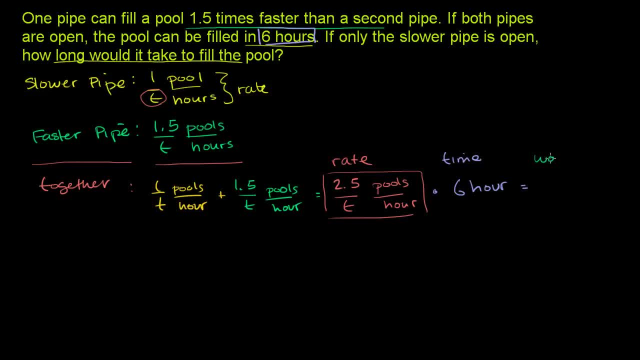 So if you get it, you get the amount of work. And I really want to emphasize this is the non-physics. If you don't know the physics definition of work, don't worry about it too much, but I don't want anyone who does know it getting confused. 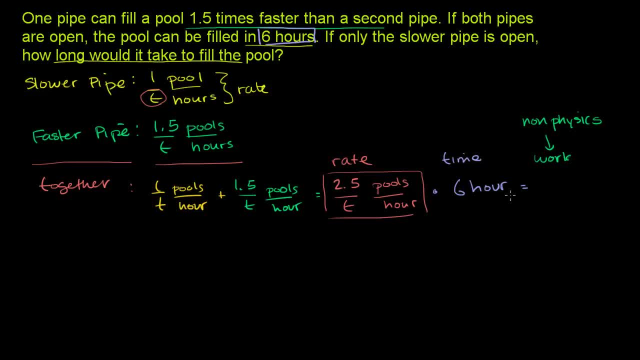 This is really just, I guess, how much of a job they can do, And so they were able to fill one pool And the units, I think, are really convenient here, because it really makes sure you're getting everything straight. So 2.5 pools per hour. 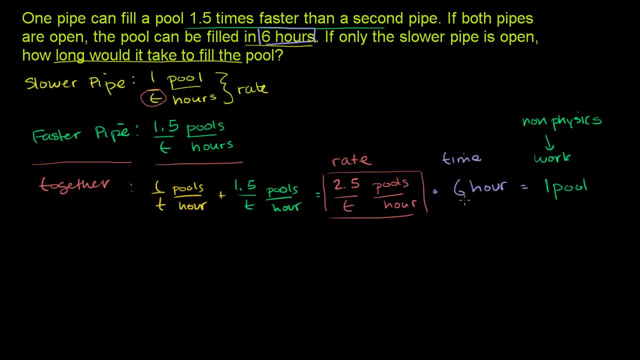 or 2.5 over T pools per hour times 6 hours gives us one pool. They give us the 6 hours right over there. That's how long it takes to fill one pool. And so now we can solve for T If we divide both sides by 6 hours. 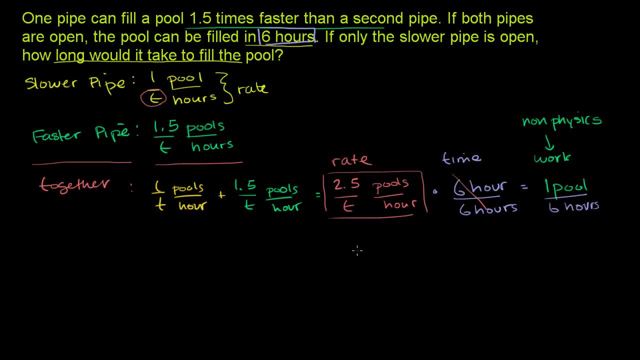 we get on the left-hand side, this cancels out. you get 2.5 over T pools per hours, I guess we could say- or pools per hour is one way to think about it- is equal to 1 over 6 pools per hour. 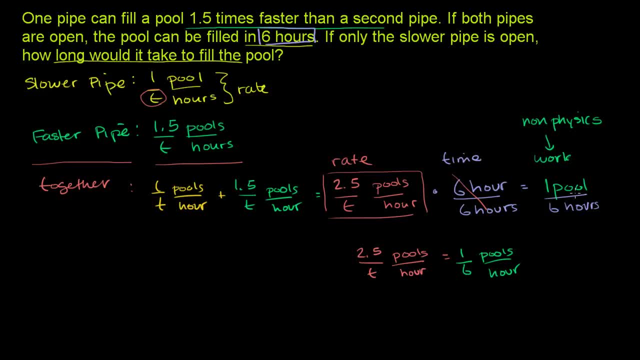 And I know I'm adding S's and taking off S's here. That's where the units start to break down a little bit. but I think you see what I'm doing. I'm just making it sound a little bit better in English. 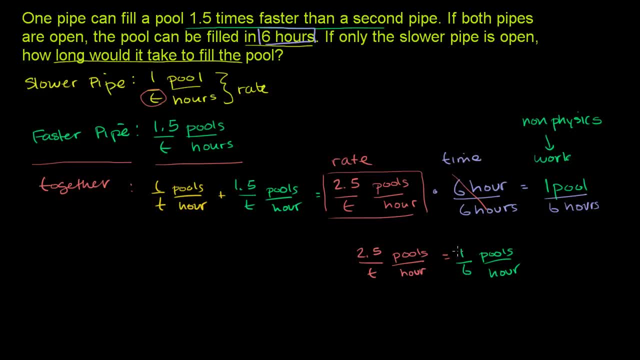 And so you have the same units on both sides. So 2.5 over T must be equal to 1 sixth. So let me write it over here. So 2.5 over T must be equal to 1 sixth must be equal. 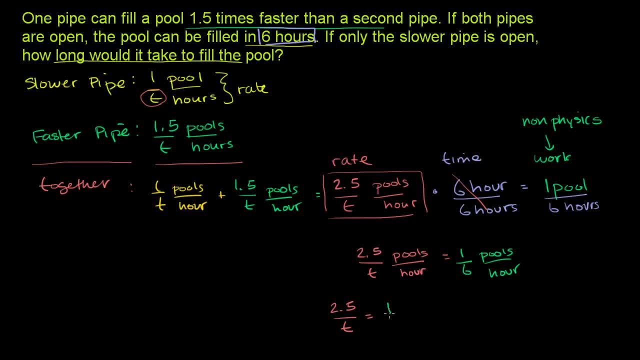 I want to do that in that green color must be equal to 1 over 6. And so we can multiply. we can multiply both sides by T and multiply both sides by 6 to get rid of the denominators there. So we're going to multiply both sides by 6. 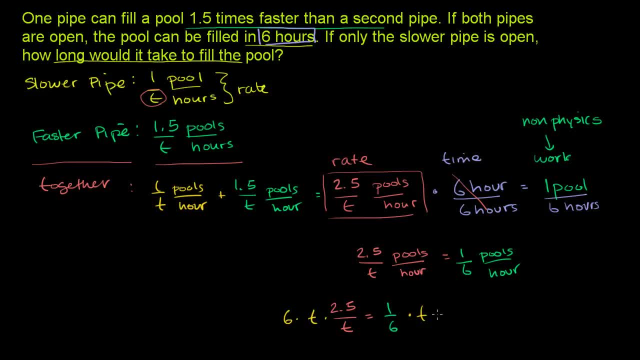 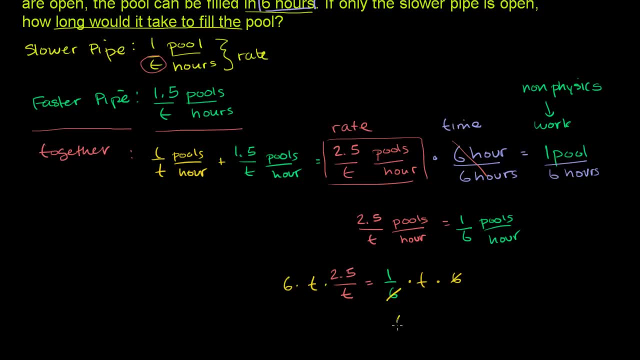 and multiply both sides by T, Both sides by T and both sides by 6.. 6 cancels with 6.. On the right-hand side, we are just left with a T- T times 1.. On the left-hand side. 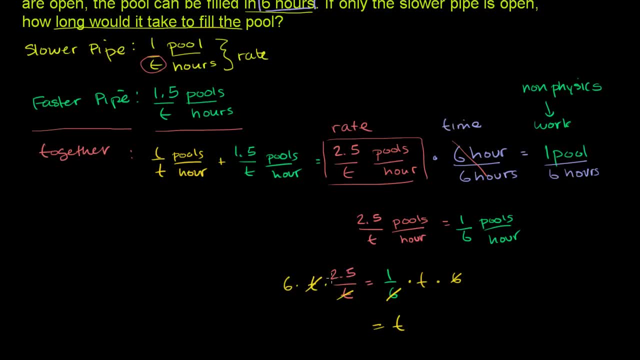 this T cancels with this T 6 times 2.5.. 6 times 2 is 12.. 6 times 1.5 is 3.. So 12 plus 3 is 15.. So T is equal to 15.. 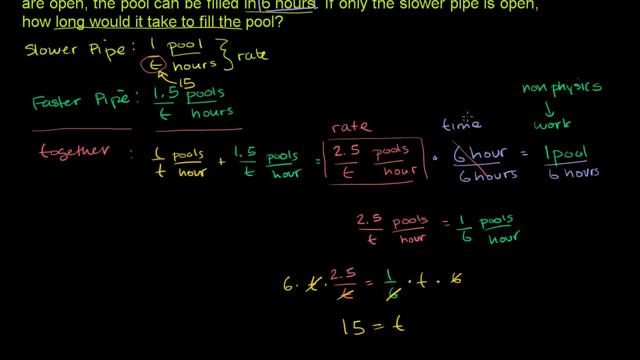 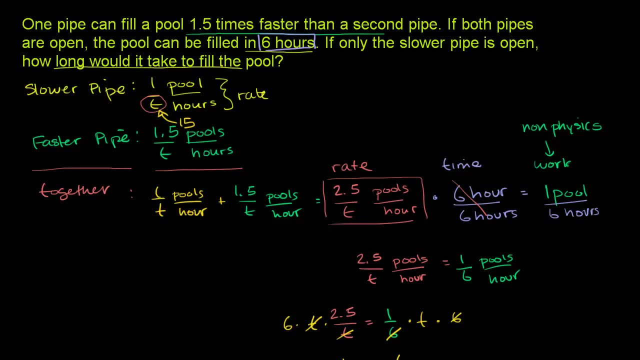 So if you go back over here you get 15 for this. So the slower pipe can fill one pool in 15 hours. One pool in 15 hours. So that answers our question. If the slower pipe is open, how long would it take to fill the pool? 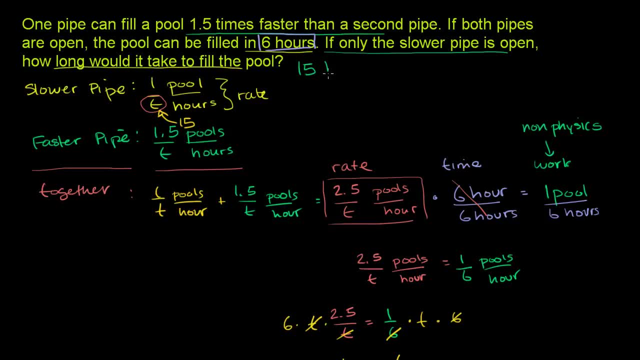 It can fill one pool in 15 hours. So the answer is 15 hours And we are done.